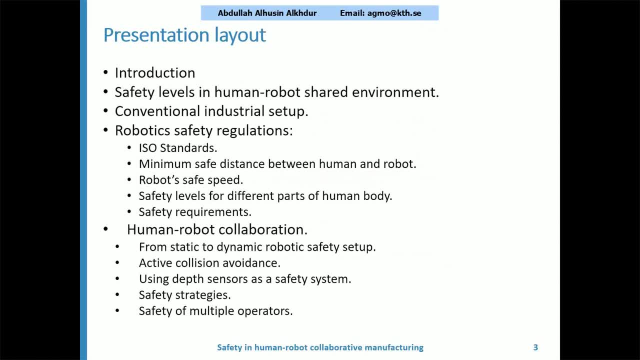 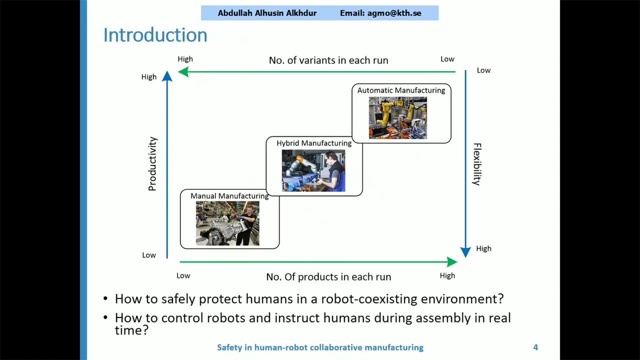 we have here at KTH is an active collision avoidance system which uses DIPTH sensors as a safety system and defining safety strategies and providing safety for multiple operators in the shop floor. so first we will try to answer the question, which is related to the first point, of what is the level of automation that we are that we need. 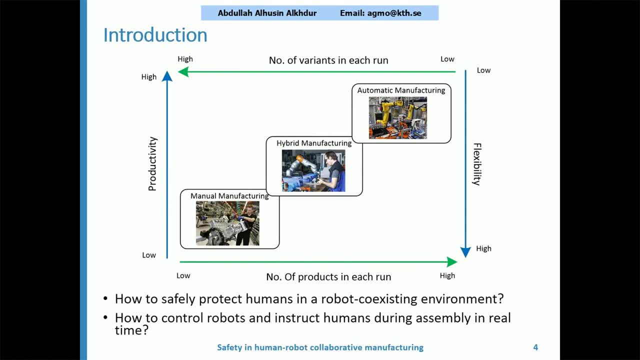 in in a, in a robotic work cell, as you can see here in the example, here the horizontal level, where you have the number of products on each run in the production line and and you have the variant on each run on the vertical direction, you will have the productivity. 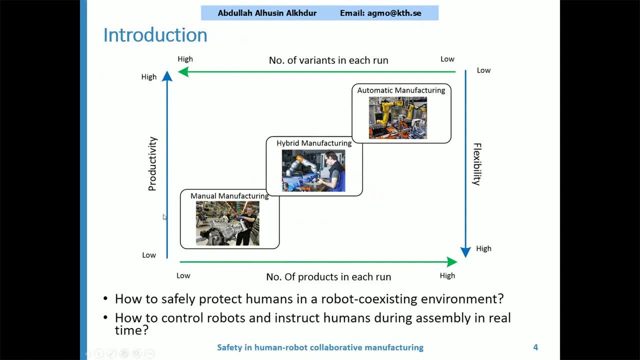 and which between low and high, and then you have the flexibility in the production line. so, basically, if you want to have low productivity and high flexibility, basically you're talking about a manual manufacturing where the number of products on each one is low and the number of variant is high, while in the 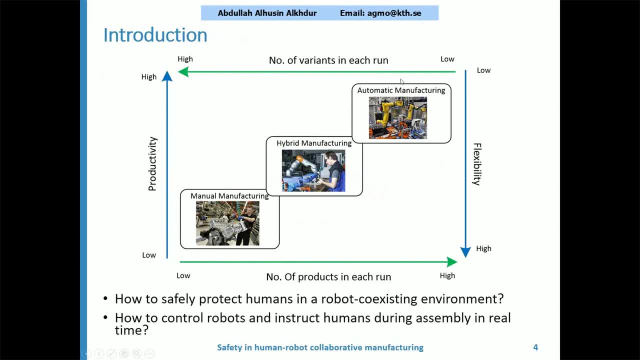 the, the, the Other direction you have in the right side, you have the far right side. automatic manufacturing. where you have the flexibility is low, The variant in each run is low, but at the same time the number of products on each. 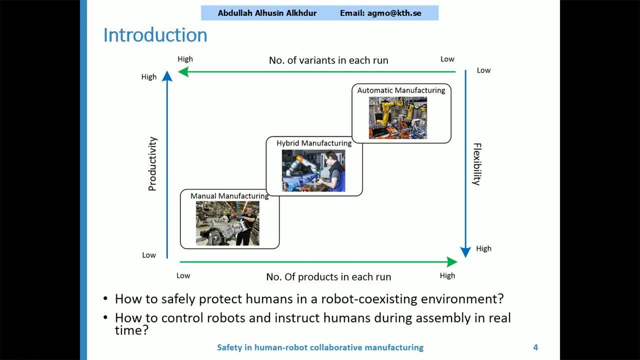 run is high, So we are talking about the mass production, So the productivity is high as well. If you want a collaborative environment where human and robot work together, then we are actually talking at the middle approach, where you have the hybrid manufacturing. 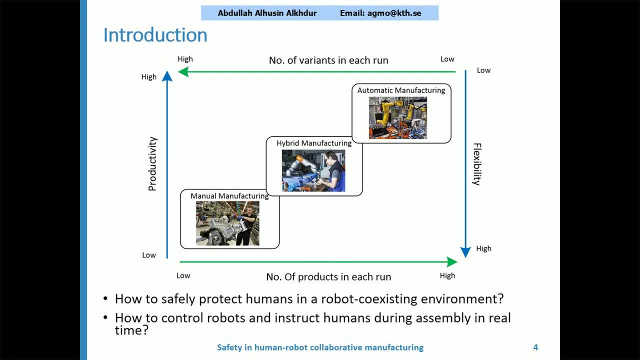 Trying to find the balance between the number of variant on each run sufficient enough and the number of product in each run is sufficient enough as well. Okay, So we are talking about the mass production which provides the balance between productivity and flexibility, as we can see in the graph here. 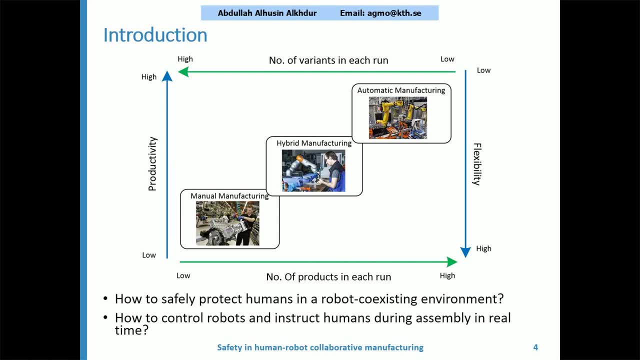 So, in addition to that, there's two main questions that if we want to go into the direction of collaborative manufacturing. the first one is how to safely protect human in a human robot coexisting environment, How to control the robot and instruct the human during an assembly operation in real 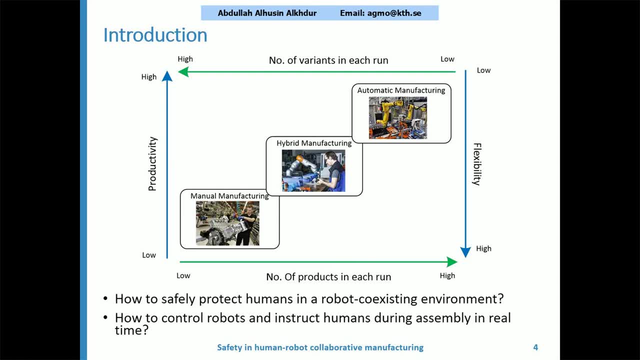 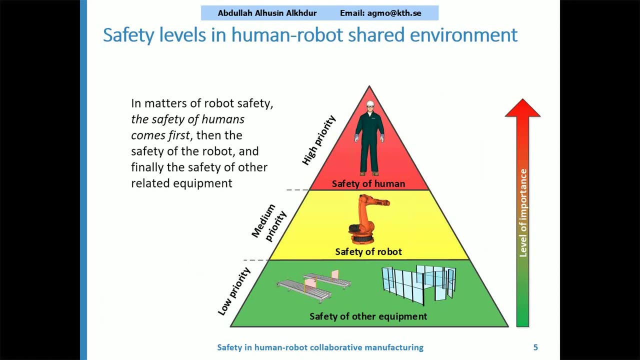 time to both avoid collision with the human and fulfill the tasks that is required from the robot. So we can take a look first on the safety level. What is the safety level in human-robot shared environment? As you can see in the graph, here you have the level of importance. 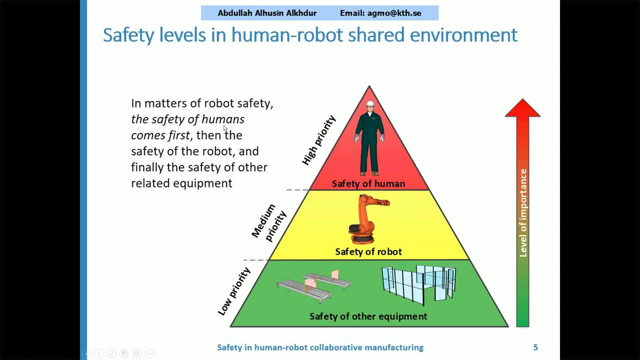 And, as you can see here, the safety of human actually comes first, with the high priority And the medium priority goes to the safety of the robot itself And then, finally, the low priority also comes first, Okay, Okay on the safety of other equipments that is used in the robotic cell. 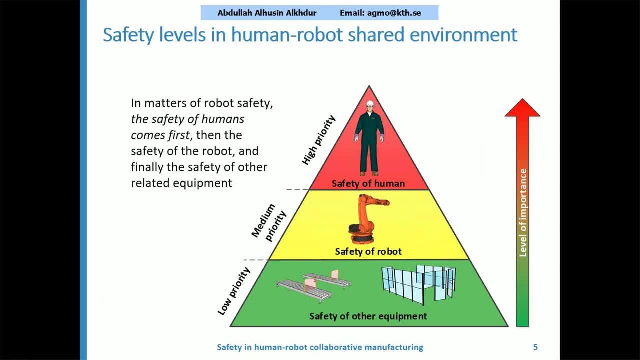 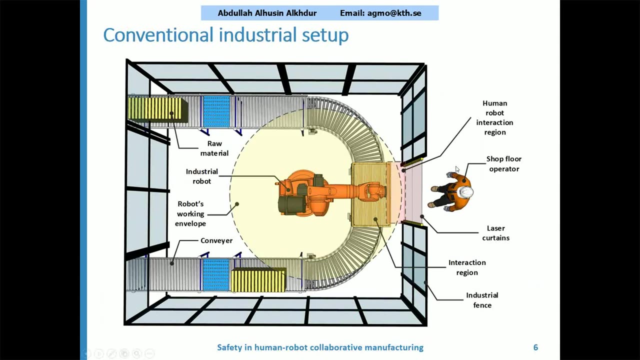 So this levels of – these levels of safety can be used as a guidelines in building any collaborative robotic work cell needed in the production line. Similarly, if we look at different work cells in any production line in a big company, most of the cases we will see that a conventional industrial setup has been installed. 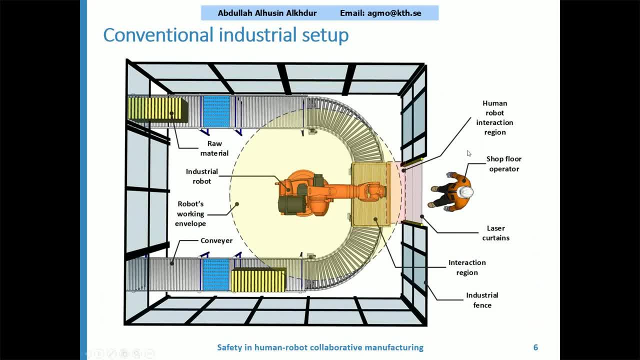 This means that the robot is actually isolated from the human with a surrounding fence, a raw material. The material comes to the robotic working envelope through a conveyor, So the robot will have access to the material. The human will have an interaction region which is controlled by a laser curtain as 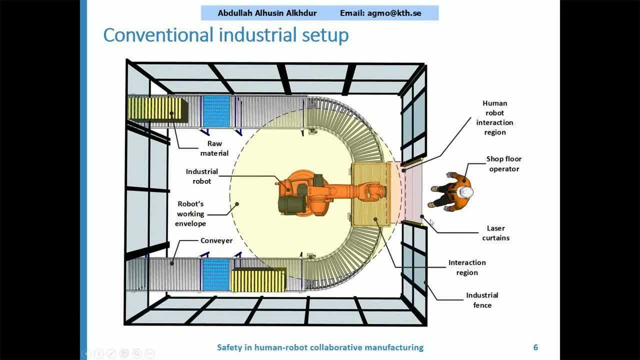 you can see in the right side of the graph, And the interaction region is where we – where the robot can share the same environment with the human At the same time. this is monitored by the laser curtain, So in case of any interruption, unexpected interruption, the robot work cell will stop. 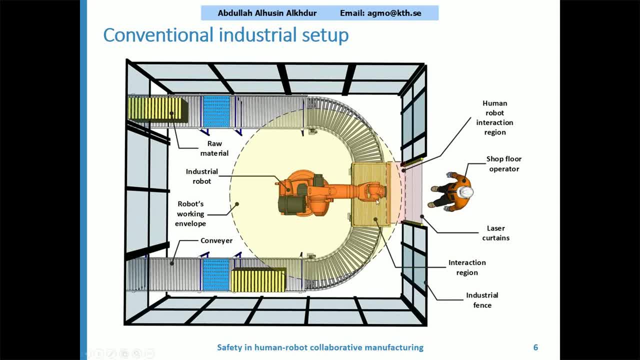 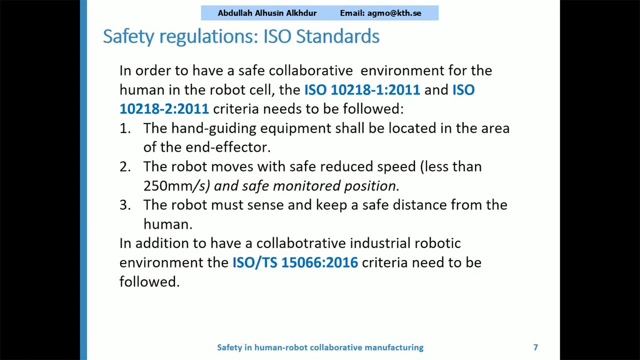 in that case, As you can see, the level of collaboration is limited In this kind of setup due to the installation of different layers of safety to fulfill the requirements, And these requirements are basically defined into different ISO standards. More specifically, there are three main safety standards currently used. 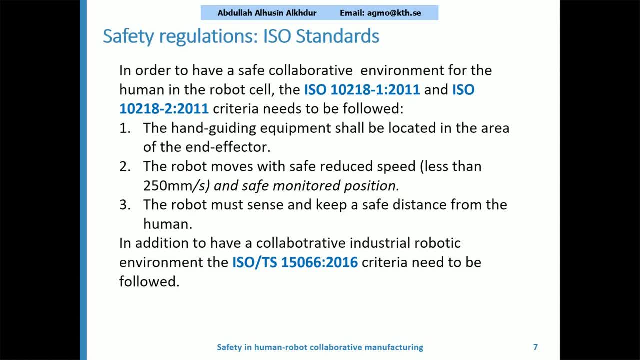 The first one is the safety standards. The second one is the safety standards. It is used for robotic and collaborative robotic. The first one is ISO 10-18,, which is two parts, actually 10-18.1 and 10-18.2.. 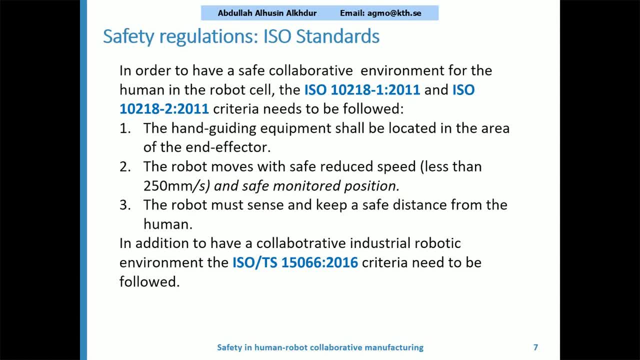 And these two standards are actually defining the criteria to how the robot works: hand guide the robot using an equipment, and this equipment will be need to be located in the area of the in defector of the robot. and another major criterion, as we can see here, is the movement of the robot, so the robot need to move in a 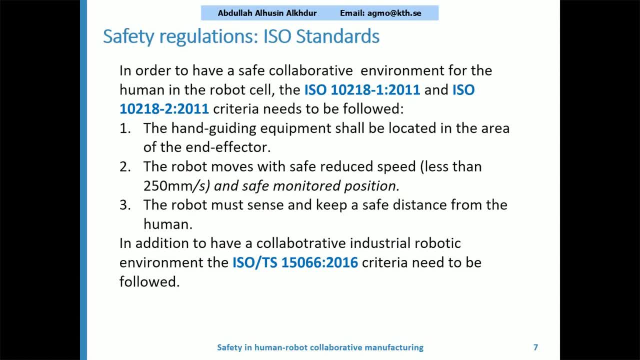 safe reduced speed which is less than 250 millimeters per second will and have a safe monitored position. a third aspect is also highlighted in in in these standards is the robot must sense and keep a safe distance from the human. so in order to you achieve that, different sensor sensors need to be installed, the robot need to. 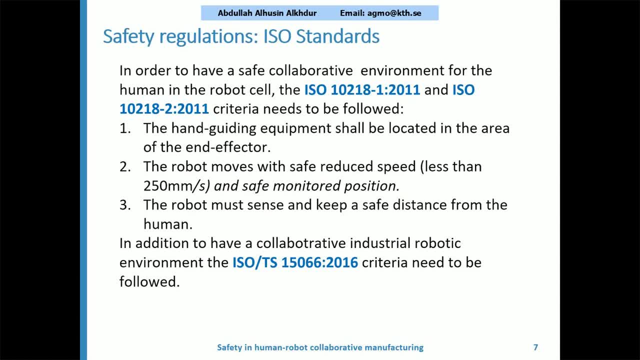 be monitored, as we will see in the following examples. in addition to that, there is also a recent standard which is at the moment is a technical specification, so it's not a standard yet. it's another form of technical specification that is available yet, which is eyesys Tieß. 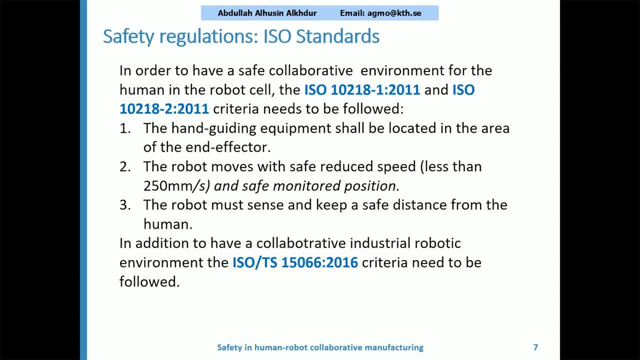 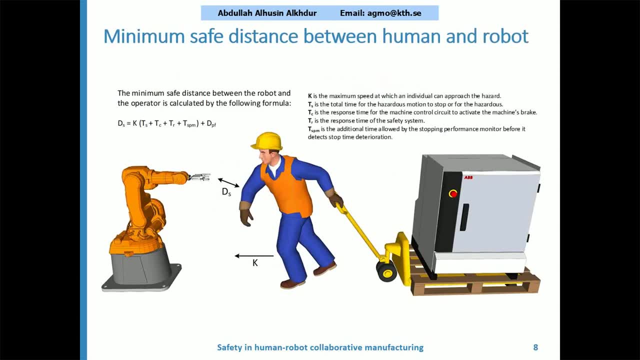 15066, and this is for the collaborative industrial robotic, which defines different Circle of acquired hypersense. aspects were highlighting the safe speed of the robot and minimum distance between the human and the robot. so if we uh look at these standards, we will find a different important formulas. the first one is uh how the 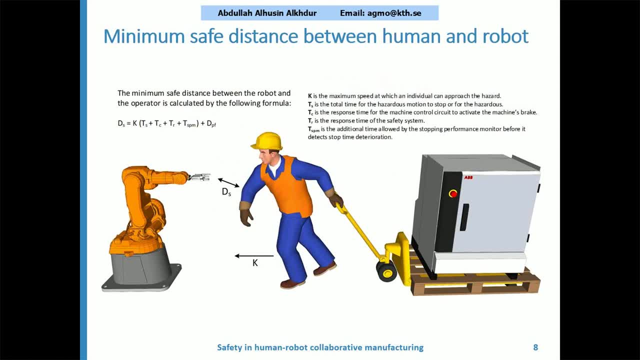 how to define the minimum safe distance between the human and the robot, which is calculated in the formula shown in the left side of this graph, um. and you can see here, um. in the example here, the operator is actually trying to approach the uh, an area which is within the reachability of the robot. so the question is how the robot need to. 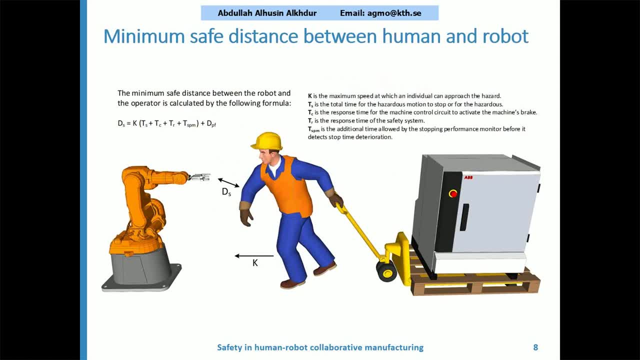 keep this distance. so the question is how the robot need to keep this distance? uh, there's a separate, several, several parameters, as you can see in the right side. one of them is k, which is the maximum speed in which the human can approach the dangerous region. ts, in this case, is the total time where the response can happen. 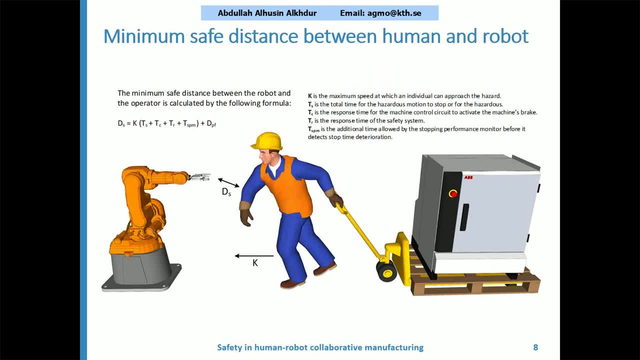 tc in this case is the response of the machine itself, the control circuit of the machine to actually stop the robot, in case of human, enter into the reachability and also parameters such as the response time for the safety system, which include sensors installed if it's a. 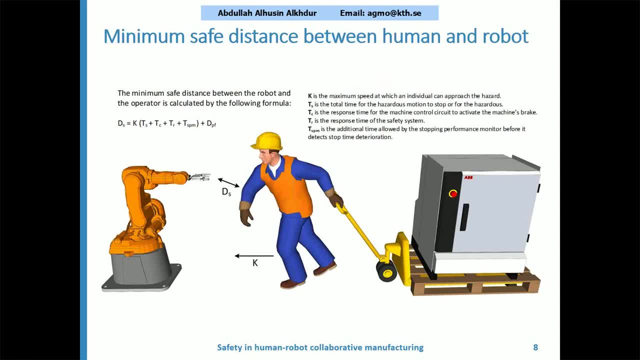 laser sensor or laser scanners, where uh if they are installed in the setup to monitor the environment. if it's a vision based, then uh, we are talking about the camera uh. response time: another parameter is his uh additional time uh to actually perform the, the stopping of the. 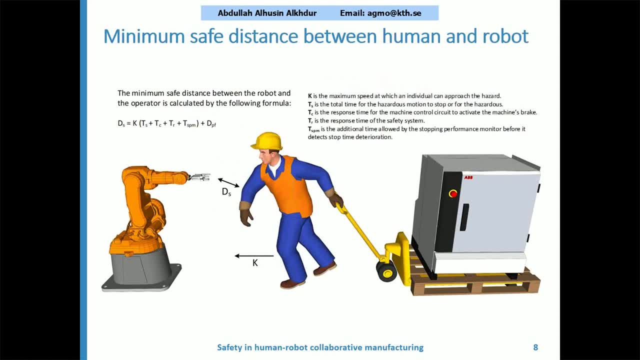 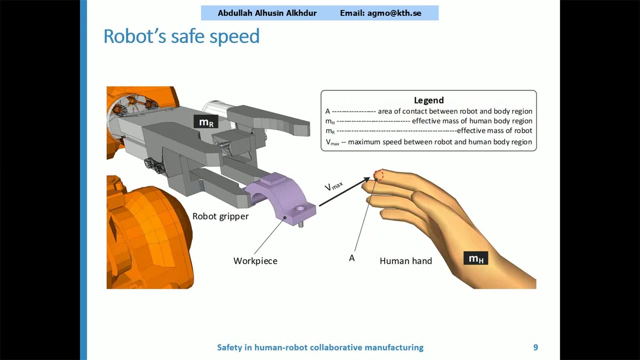 of the robot itself. so these are. this kind of formula is actually defined in the standard, with the details on how can be implemented. another aspect or another, another point that need to be taken into consideration is the robot safe speed, which is also defined in the standard, and a different parameters actually. 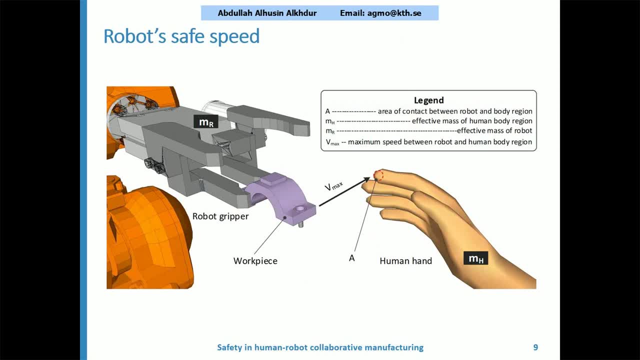 define the that speed that is needed. the first one is where the area of contact between the robot and the human body and also the effective mass of the human body part- either it's an hand or an arm, for example, or the shoulder of the operator, and so on- and also the effective mass of the robot need to be. 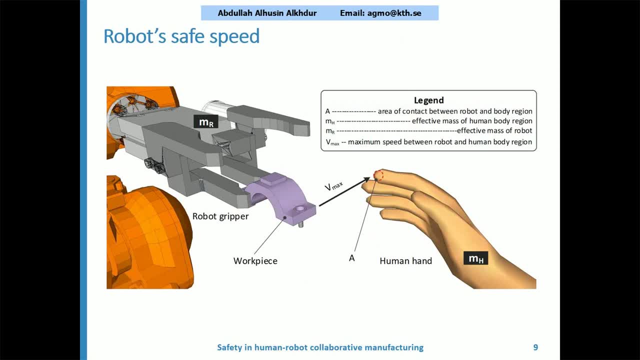 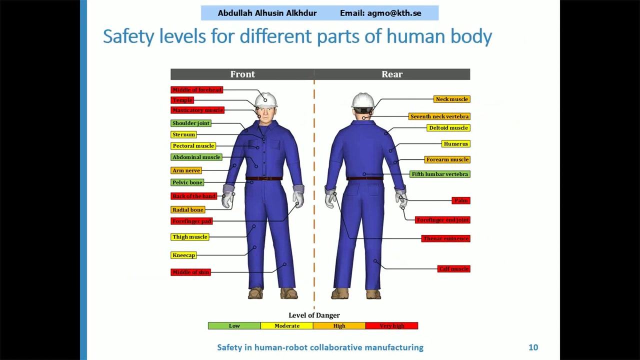 taken into consideration in determining the safe speed as well as the maximum speed between the robot and human body in that aspect. so if we look at the different parts of the human body, which is an important factor as well in the determining the level of danger, and also the effective mass of the human body and so on, and also the effective mass, which 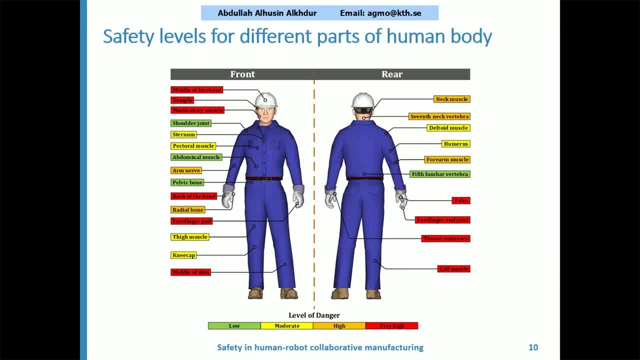 and as well as the parameters for the safe robot speed. if you look at this example here, we can see different parts actually have different levels of danger, parts like the head of the robot், And so we keep it as an example here where the ஆN and that is different levels. 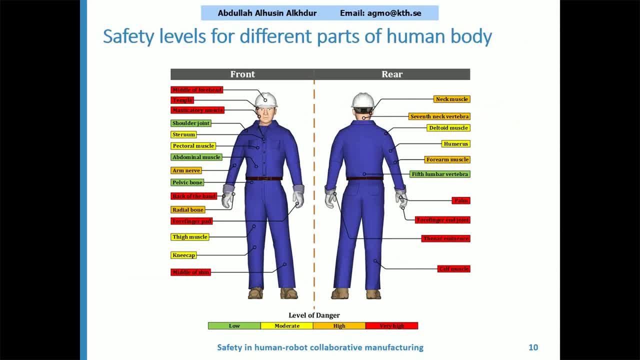 of danger. so if we look at the example here we can see that different maps are actually have different levels of danger conditions and we have to значит that if you lower here the overall distance in each case yep of chance because all kinds of changes operator and the arms, more specifically the, the hands of the operator, are in a 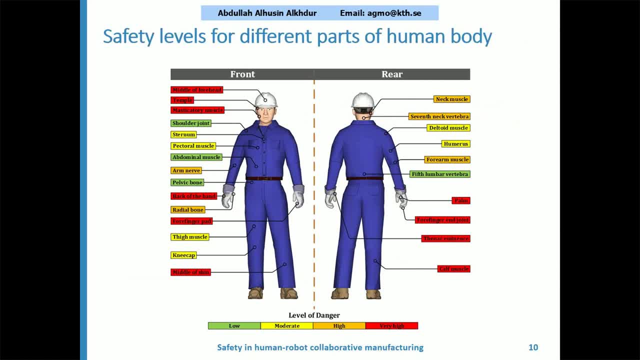 high level of danger, while parts such as the, the shoulder, the, the core of the body of the operator, is in a lower level of danger. these are basically defining the standards and based on the statistical analyses of previous cases of accidents that might happen and studying how the mass of each part of 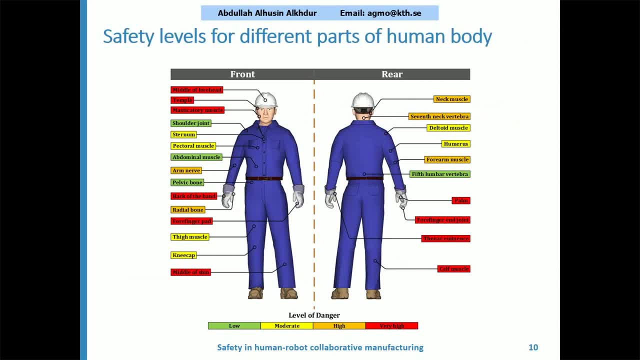 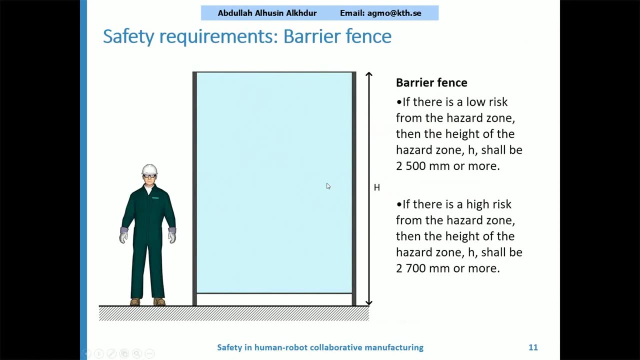 the human body is distributed, so this is also need to be considered in the preparation of a collaborative setup. so if we look at the safety requirements based on the standards, there's a different aspects that need to be taken into consideration. the first level of protection that we can see in a protected conventional robotic work some is 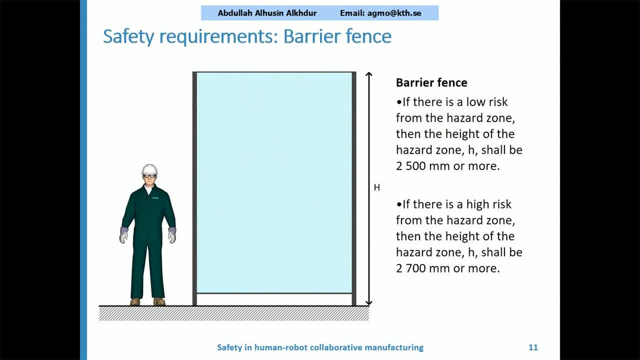 Glasgow barrier fence: cook using this: apply 거는 Authority law barrier fence: okay, the low-risk to be in that hazard region, then the height of the of the fence need to be around two, two and a half meter or more. and if, in the other case, if we have a 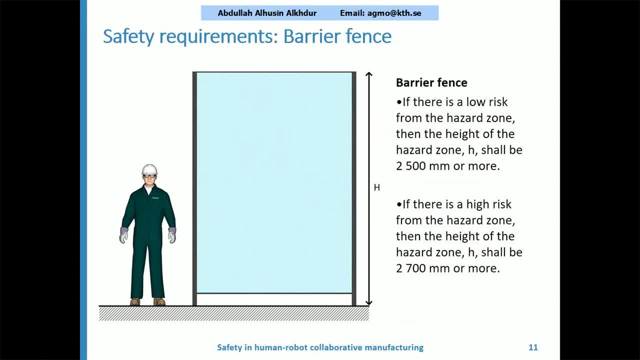 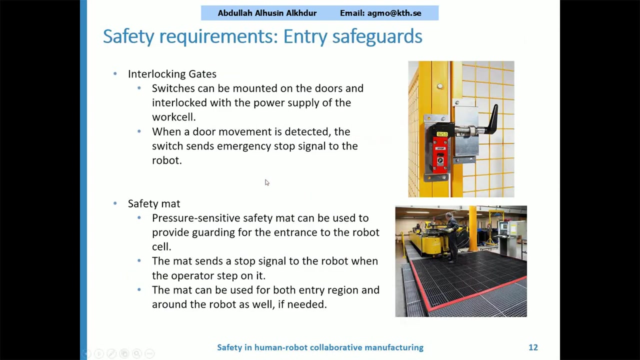 high risk of hazard zone, then the height need to be elevated to 2.7 meters or more to be to guarantee a safe fence so the operator can work in that environment. there's also different aspects of safety. the other aspect is the entry safeguards. there's different approaches. 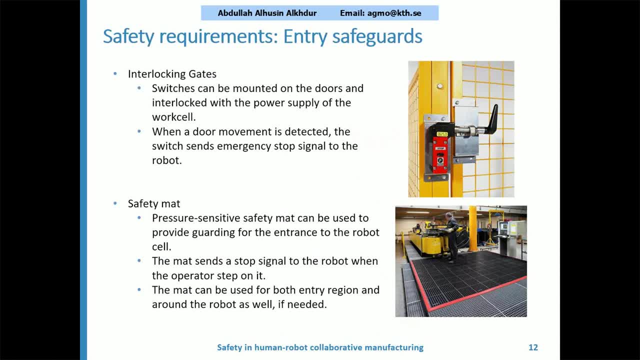 in having an entry to the robotic cell, which actually hesitate in some cases, is the interaction between the human and the robot. the first one is the case of interlocking gates, So this can be seen in the production line, where switches can be mounted on the doors. 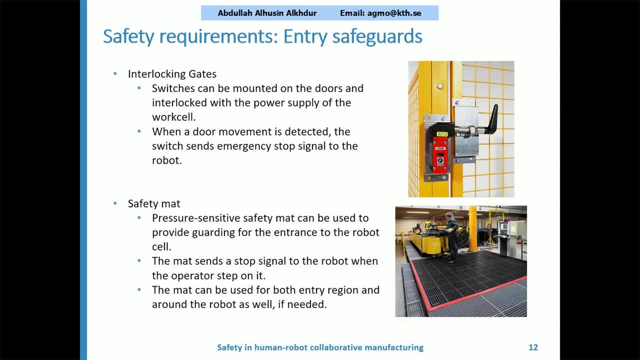 and interlocked with a power supply from the work cell, And when the door movement is detected, which in this case, someone opened the door- then the switch sends an emergency stop signal to the robot and the whole work cell will shut down. Another approach is to have a safety mat which is a pressure sensitive, as you can. 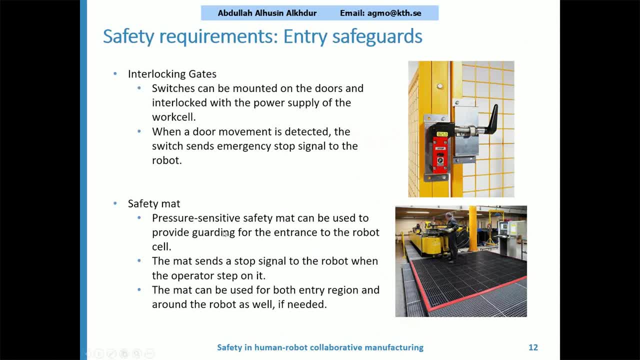 see in the lower part of the figure, in the lower part, where you have the pressure sensitive safety mat, And it can provide a guarding for the entrance of the robot cell. The mat sends a stop signal similar to the interlocking gates to the robot, when the 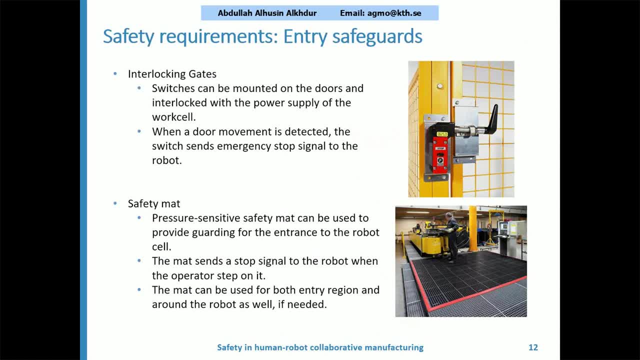 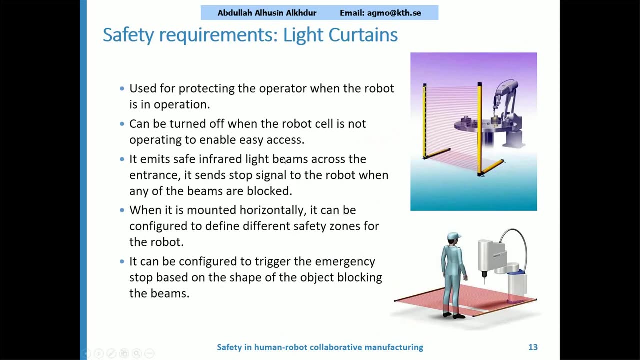 operator steps on it, And also the mat can be used for both entry region and around the robot as well, if it's needed. Next slide, please. Another safety level, or could be also an entry safeguard, is the light curtain, As you can see the example in the first figure, in the upper figure, where you have the light. 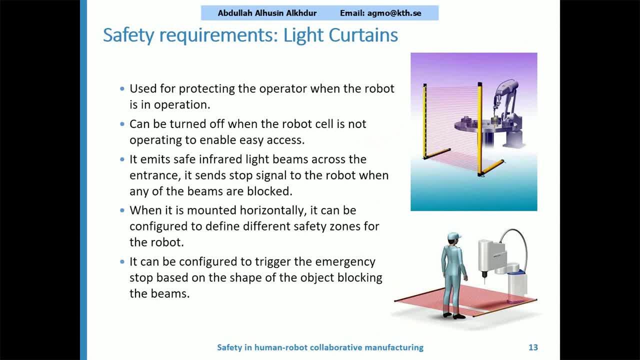 curtain is actually mounted on the vertical setup which is used for protecting the operator when the robot is in operation, And they can be turned off when the robot cell is not operating to enable easy access, For example, in the case of maintenance and so on. 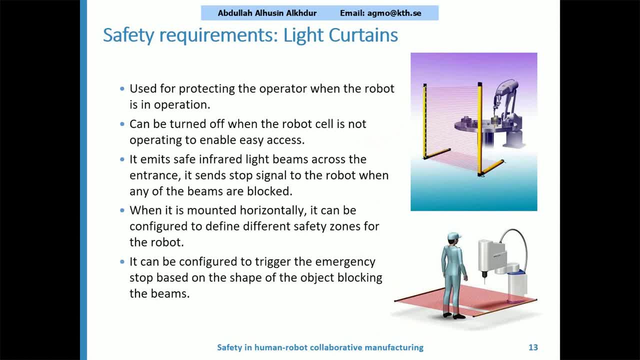 So basically it works on emitting a safe infrared light beam across the entrance. It sends a stop signal when the beam is interrupted And the stop signal is then sent to the operator. Next slide, please. The emergency stop signal is sent to the robot and basically shut down the robotic work cell. 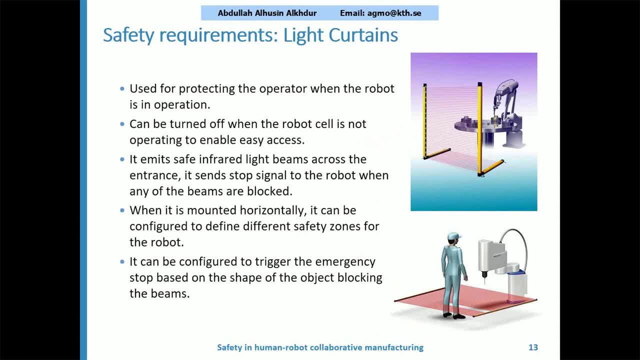 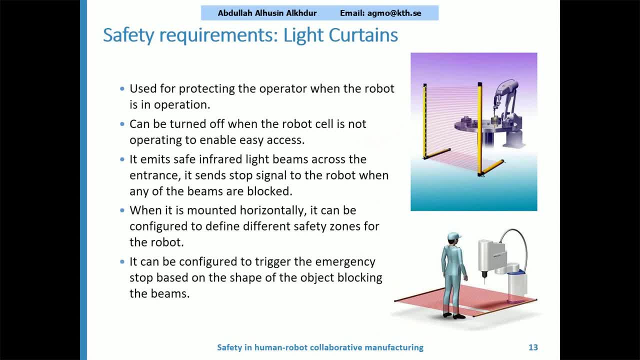 So this is the basic of the safety zones for the robot, And so it can be configured to trigger the emergency stop based on the shape of the object blocking the beam And also the distance between the human and the robot. So in that horizontal setup, the zones can be defined as well as having information about. 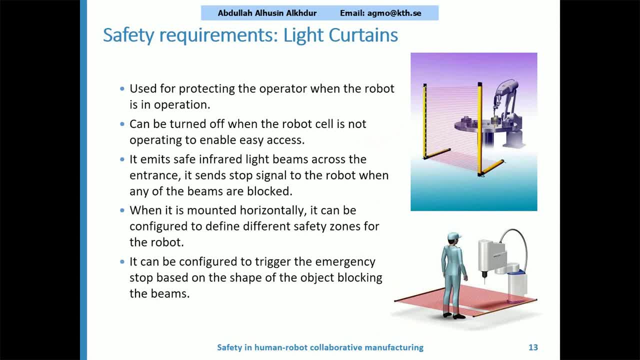 the shape of the object. Next slide, please: a moving AGV. if it enter to that light curtain and if the if they are defined in a way that doesn't interrupt the robot, then that will not trigger emergency stop. well, if the human enter to that and block, block these light. 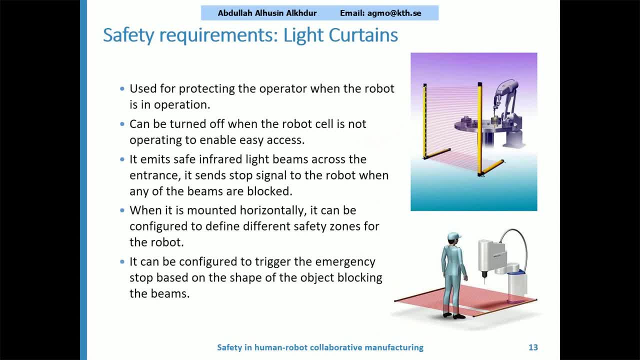 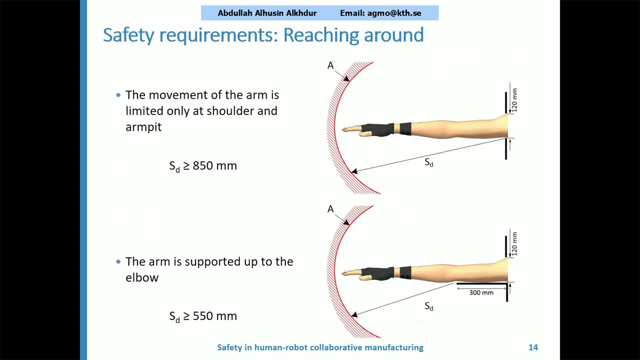 curtains based on the shape, though the system can know that then human enter to that loop. therefore it has the highest safety priority. then it will basically slow down the robot or completely stop the robot as emergency stop. another aspect for the safety requirement is the reaching around this. 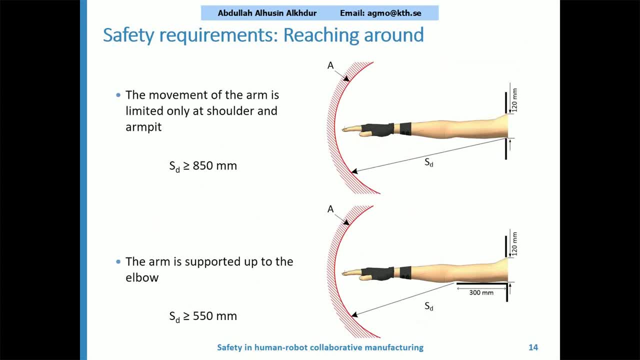 is applied when we have a fence that is lower than the operator height around the robot. and if we have, then in that case we need to have a distance between the fence itself and the robot, and if we have, then in that case we need to have a distance between the fence itself and the robot. 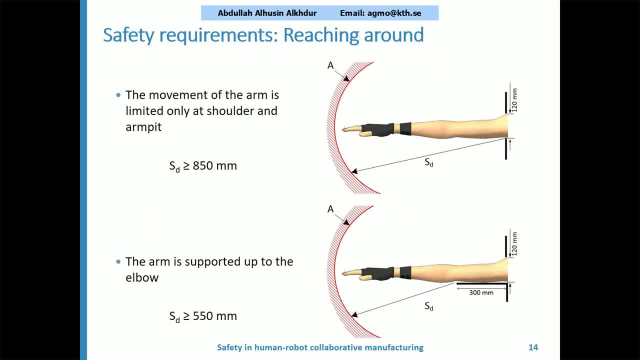 working envelope and basically this gap or this space is defined by the parameter SD in the in the figure here, where a here in this case is hazard zone. so in the first example where we have, the movement of the arm is limited only to the shoulder and armpit. 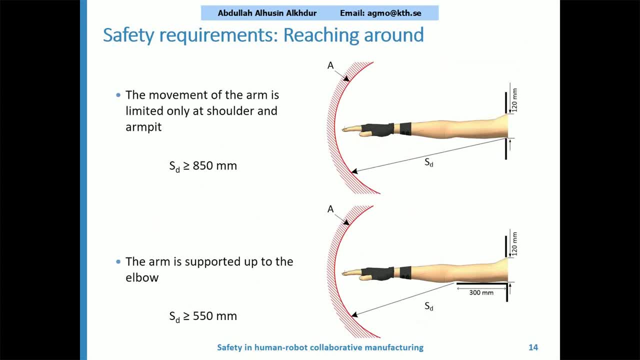 and in the second example where we have the arm is supported up to the elbow. so in the first upper figure we have the SD need to be around 850 millimeters or more, and in the lower one could be 550 millimeters or more in that case, which is? 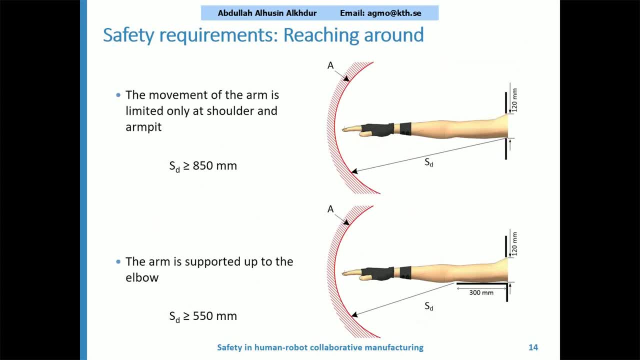 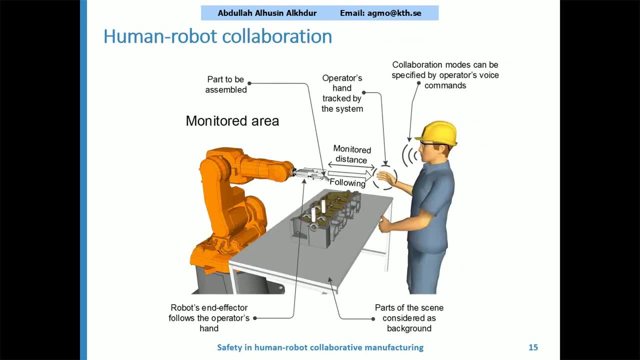 the safe distance in in the lower one could be 550 millimeters or more in that case, which is the safe distance in in that in that figure. so, in order to actually have a collaborative environment, the safety requirements that are mentioned in the previous slides sort of create an. 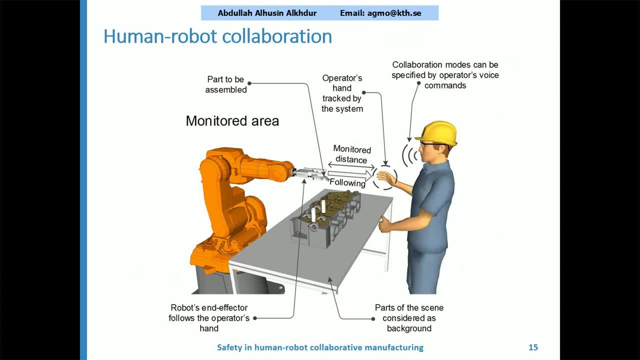 obstacle to this kind of close collaboration. therefore, we can see now there is a new paradigm in the industrial robotics using. there is a new paradigm in the industrial robotics using and collaborative robots, or using an equipment that can be installed to and collaborative robots, or using an equipment that can be installed to. 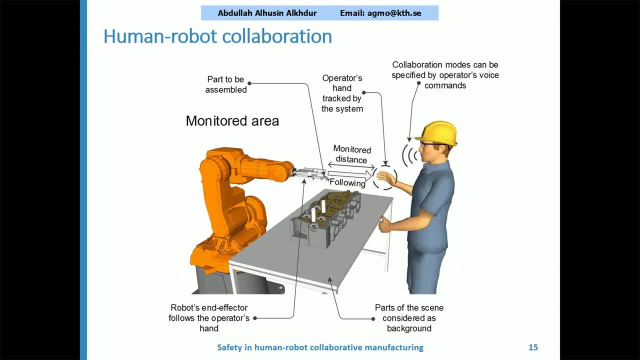 provide this close collaboration with different types of sensors to guarantee. provide this close collaboration with different types of sensors to guarantee a safe interaction between the human and the robot. so, if we look at the, the, the- a safe interaction between the human and the robot. so, if we look at the, the, the- 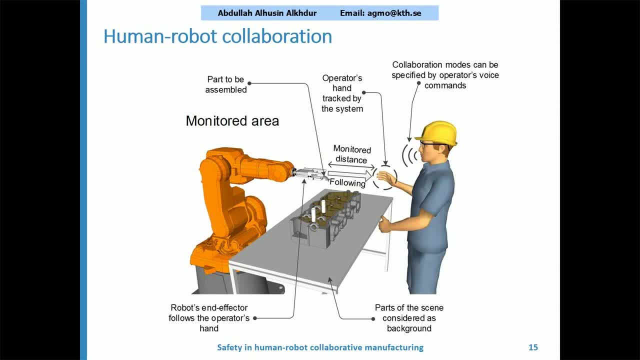 concept behind the human robot collaboration concept behind the human robot collaboration. we can see the example here where a robot is actually. we can see the example here where a robot is actually. we can see the example here where a robot is actually monitored through different sensors and the. 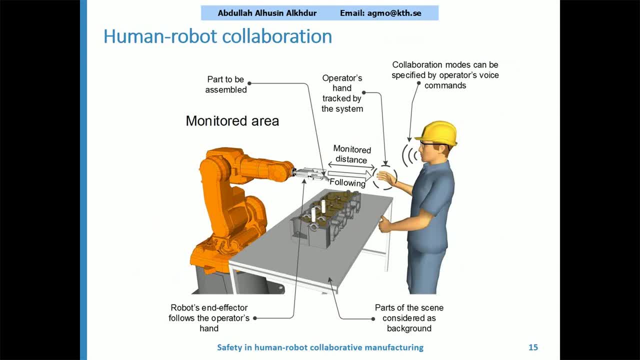 monitored through different sensors and the monitored through different sensors and the operator can use the voice command to operator, can use the voice command to operator, can use the voice command to facilitate a collaboration mode which is facilitate a collaboration mode which is facilitate a collaboration mode which is, in this case, hybrid assembly, where the 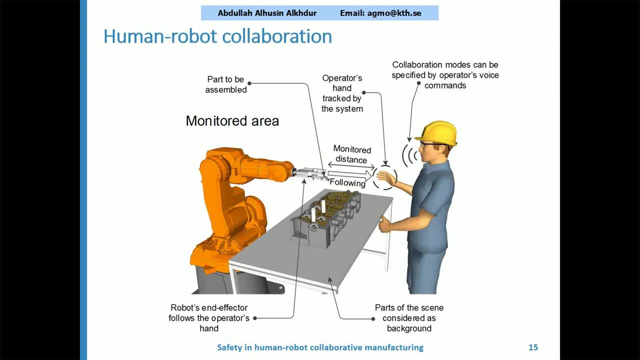 in this case, hybrid assembly, where the- in this case, hybrid assembly, where the robot is helping the operator to assemble, robot is helping the operator to assemble, robot is helping the operator to assemble different parts of an different parts of an different parts of an engine. the safety system keeps the safe. 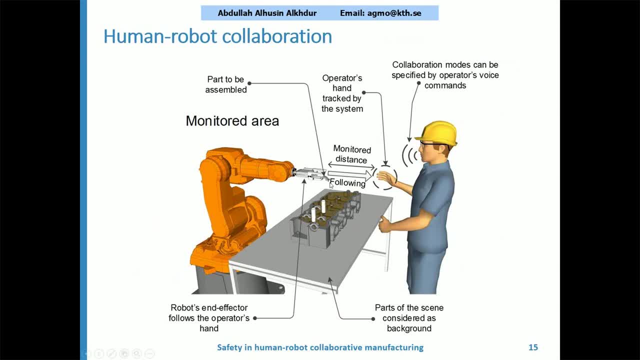 engine. the safety system keeps the safe engine. the safety system keeps the safe distance between the human and the robot, distance between the human and the robot, distance between the human and the robot. at the same time trying to follow the. at the same time trying to follow the. 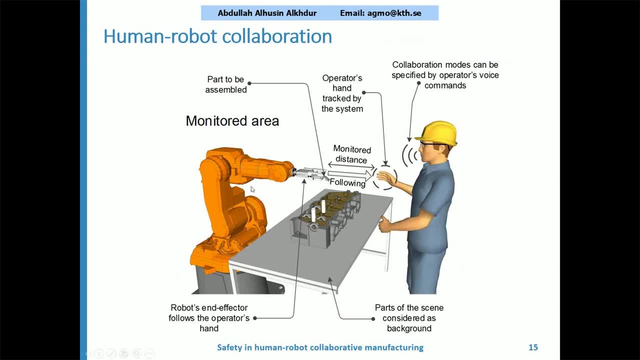 at the same time trying to follow the operator hand with the safe robot speed operator hand, with the safe robot speed operator hand with the safe robot speed. so the end effector of the robot follow. so the end effector of the robot follow, so the end effector of the robot follow the operator hand and hands in the 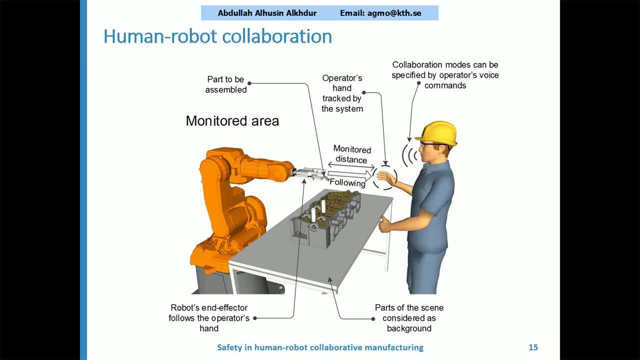 the operator hand and hands in the, the operator hand and hands in the different parts that need to be different parts that need to be different, parts that need to be assembled, so the operator can perform the assembled, so the operator can perform the assembled, so the operator can perform the assembly. so this actually in that kind. 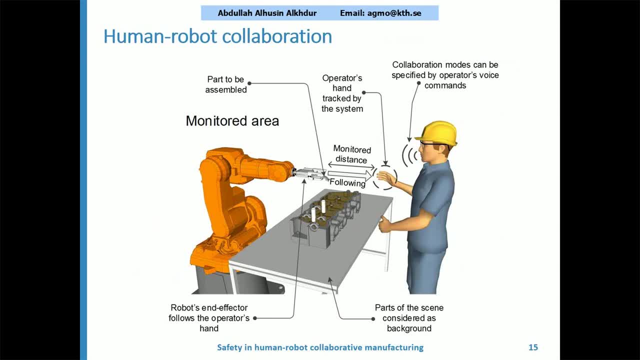 assembly. so this actually in that kind assembly, so this actually in that kind of scenario. it's fulfilling the of scenario. it's fulfilling the of scenario. it's fulfilling the definition for a collaborative human definition, for a collaborative human definition, for a collaborative human robot manufacturing environment. so as we 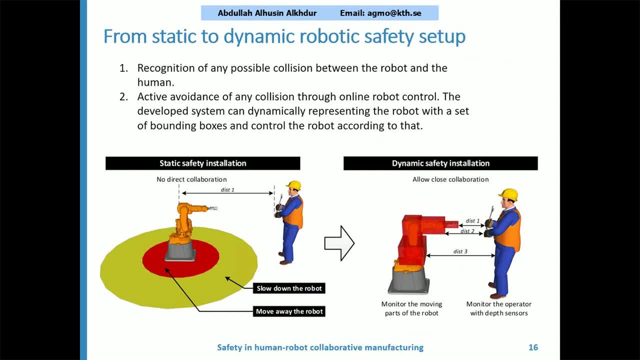 robot manufacturing environment. so, as we robot manufacturing environment, so as we can see from the previous example, can see from the previous example, can see from the previous example, this is basically moving from the. this is basically moving from the. this is basically moving from the paradigm of having a static safety. 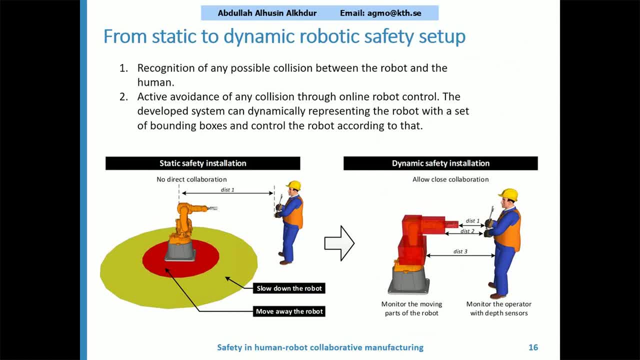 paradigm of having a static safety paradigm, of having a static safety installation into a dynamic safety installation, into a dynamic safety installation, into a dynamic safety installation. in that case, the as in the installation. in that case, the as in the installation. in that case, the as in the conventional robotic cell where we have 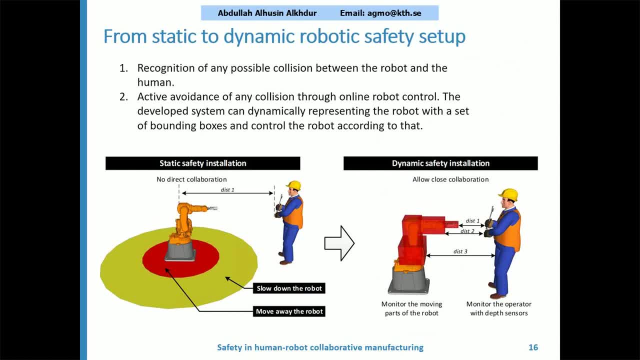 conventional robotic cell. where we have conventional robotic cell, where we have the static safety installations, there is the static safety installations, there is the static safety installations. there is no direct collaboration because it might no direct collaboration. because it might no direct collaboration because it might be possible to define a different zones. 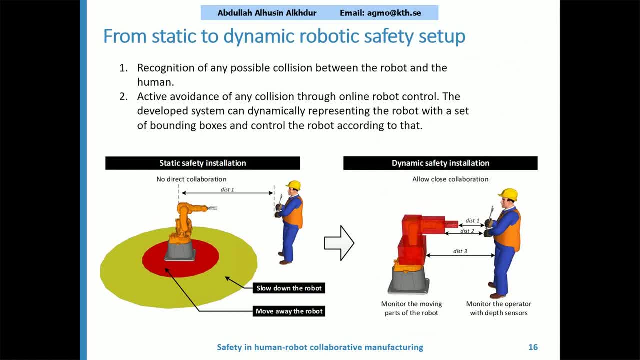 be possible to define a different zones, be possible to define a different zones around the robot to slow down the robot around the robot. to slow down the robot around the robot. to slow down the robot and move away the robot and so on. but and move away the robot and so on, but. 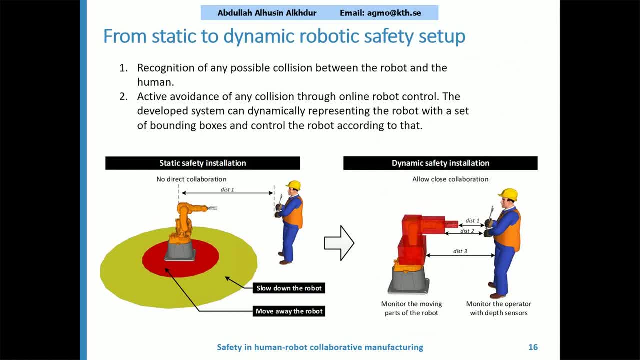 and move away the robot and so on. but this level of collaboration, it is usually this level of collaboration. it is usually this level of collaboration. it is usually limited because the system needs limited, because the system needs limited, because the system needs to keep a high distance between the human. 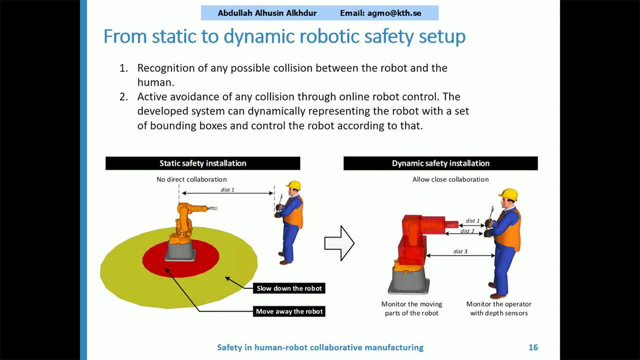 to keep a high distance between the human, to keep a high distance between the human and the robot, to avoid any potential and the robot to avoid any potential and the robot to avoid any potential collisions. while in the dynamic collisions, while in the dynamic collisions, while in the dynamic safety installation, it is actually allow a 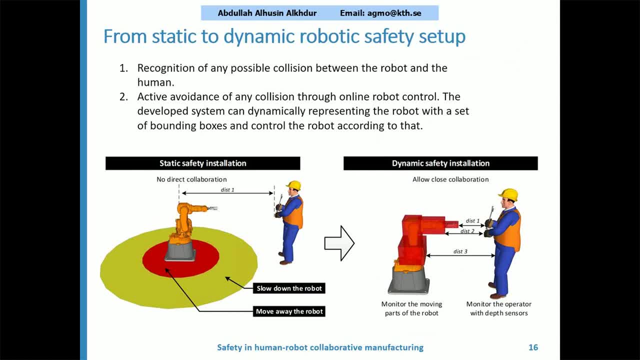 safety installation. it is actually allow a safety installation. it is actually allow a close collaboration. so this is achieved, close collaboration. so this is achieved, close collaboration. so this is achieved by the two points that is shown here, by the two points that is shown here, by the two points that is shown here, which the first one is recognizing any 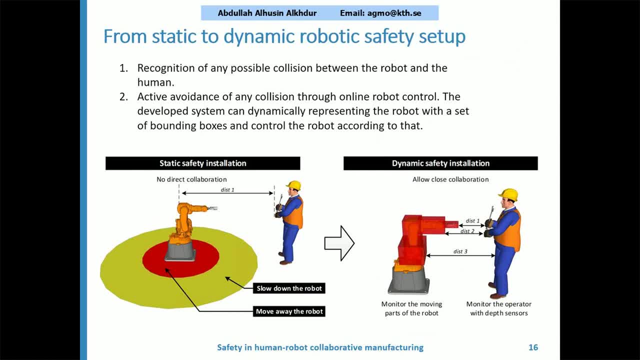 which the first one is recognizing any, which the first one is recognizing any possible collisions between the robot, possible collisions between the robot, possible collisions between the robot and human, and actively avoid any and human and actively avoid any and human and actively avoid any collision through an online robot. 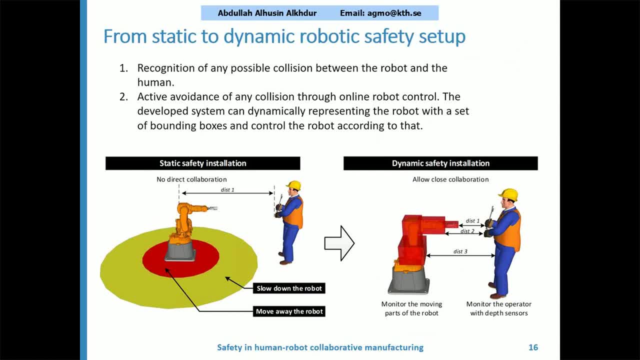 collision through an online robot. collision through an online robot. control. this control, this control, this kind of setup is dynamically representing the robot with: kind of setup is dynamically representing the robot with. kind of setup is dynamically representing the robot with a set of bounding boxes, as we can see in. 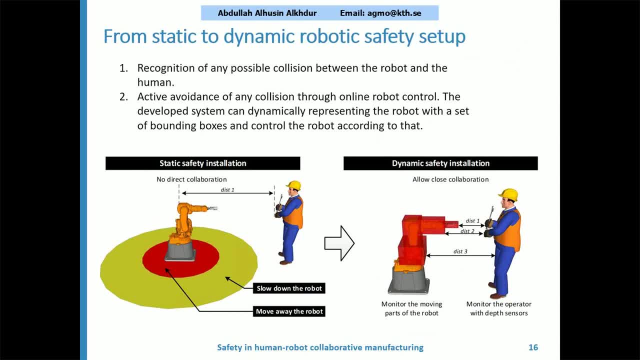 a set of bounding boxes, as we can see in a set of bounding boxes, as we can see in the right figure, the figure in the right, the right figure, the figure in the right, the right figure, the figure in the right side, with different distances, and these side with different distances. and these 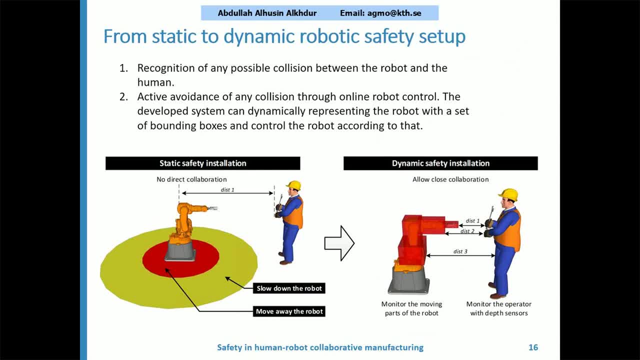 side with different distances, and these distances are actually monitored through. distances are actually monitored through. distances are actually monitored through the sensors and controlling the robot, the sensors. and controlling the robot, the sensors. and controlling the robot according to that: to keep this distance. according to that, to keep this distance. 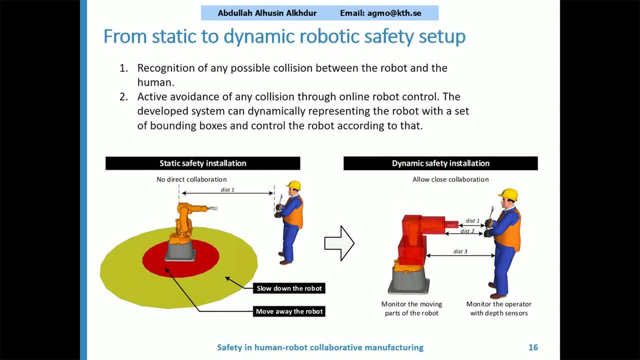 according to that, to keep this distance in an accepted level in this example, in an accepted level in this example, in an accepted level in this example, the monitor is that the robot is actually the monitor, is that the robot is actually the monitor, is that the robot is actually monitored through the joint values and 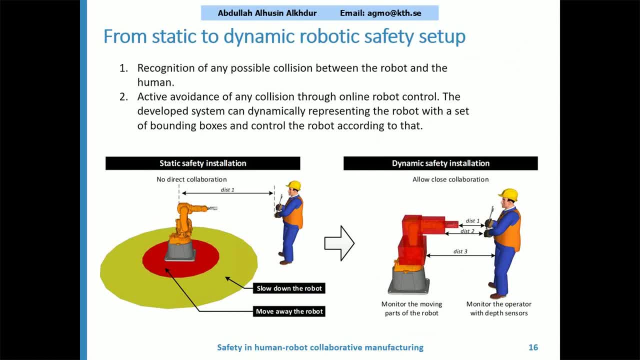 monitored through the joint values and monitored through the joint values and the CAD module of the robot, while the, the CAD module of the robot, while the- the CAD module of the robot, while the operator or the human are actually operator or the human are actually operator or the human are actually monitored through the depth sensors and. 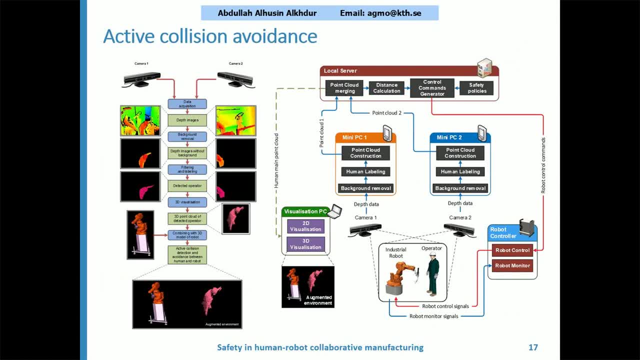 monitored through the depth sensors and monitored through the depth sensors. and this is how, this is how. this is how an approach we have developed here at an approach we have developed here at an approach we have developed here at KT edge- that is actually facilitate this KT edge, that is actually facilitate this. 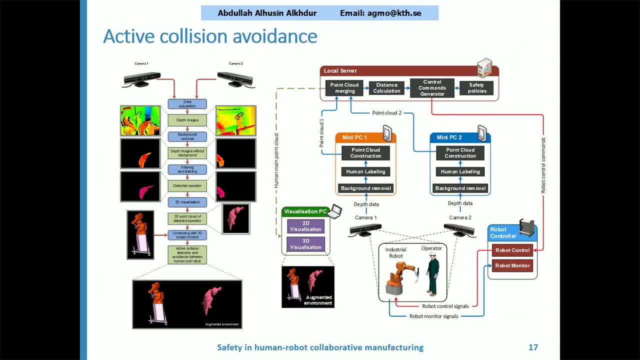 KT edge. that is actually facilitate this kind of collaboration. we have used for kind of collaboration. we have used for kind of collaboration. we have used for as a depth sensors. we have used kinetic as a depth sensors. we have used kinetic as a depth sensors. we have used kinetic sensors. that is basically capturing the 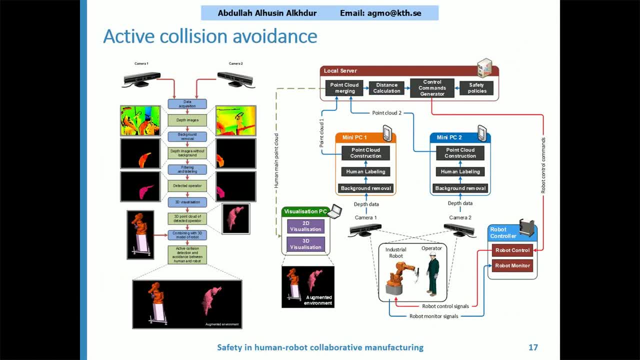 sensors. that is basically capturing the sensors. that is basically capturing the depth information from the scene. depth information from the scene. depth information from the scene, determining which are the static parts, determining which are the static parts, determining which are the static parts in the scene, in the scene. 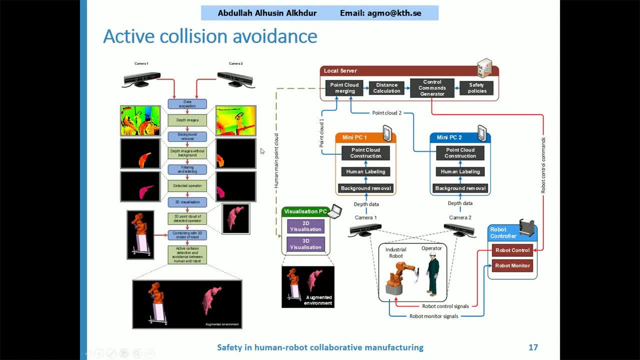 in the scene, removing these static parts. so it consider removing these static parts. so it consider removing these static parts, so it consider that these parts as a background and that these parts as a background, and that these parts as a background, and then, when the human enter into the loop, 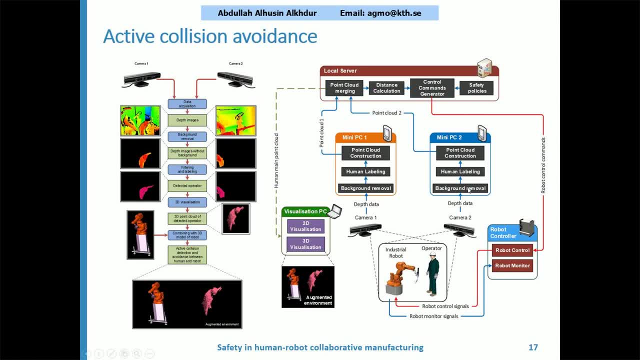 then when the human enter into the loop, then when the human enter into the loop, it will be detected as moving object or it will be detected as moving object, or it will be detected as moving object or as a human with different angles of, as a human with different angles of. 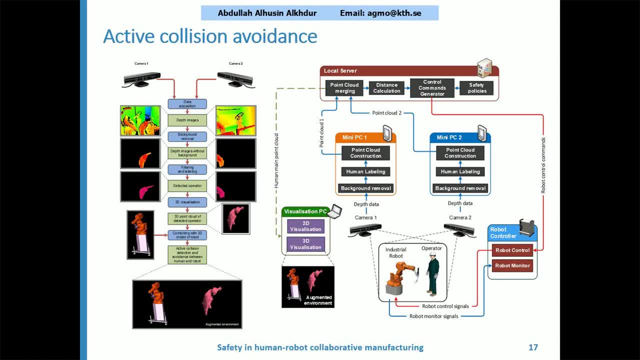 as a human, with different angles of capturing, capturing, capturing which allows us to fuse this information, which allows us to fuse this information, which allows us to fuse this information from different kinetic sensors. in this, from different kinetic sensors in this, from different kinetic sensors. in this example, you can see two kinetic sensors. 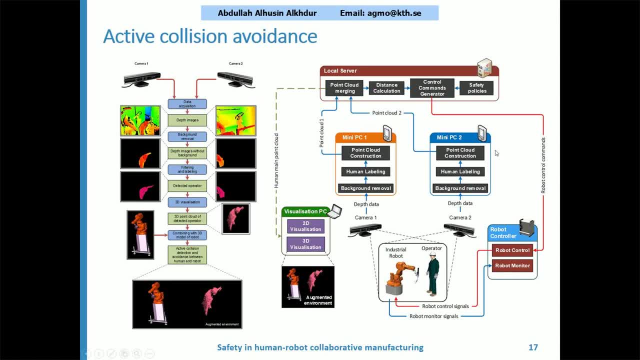 example, you can see two kinetic sensors. example: you can see two kinetic sensors that are connected to our two mini PCs. that are connected to our two mini PCs. that are connected to our two mini PCs and in the local server they are the and in the local server they are the. 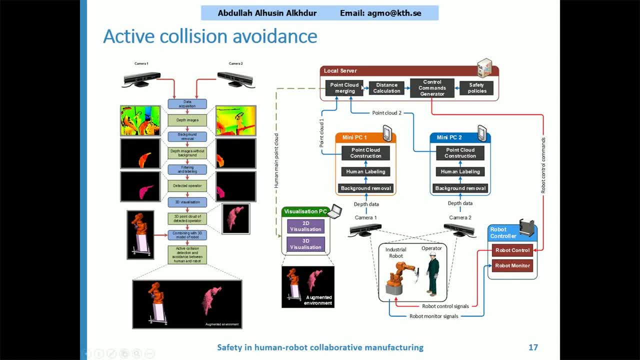 and in the local server they are, the point cloud are fused together and the point cloud are fused together and the point cloud are fused together and the distance between the human and the robot, distance between the human and the robot, distance between the human and the robot are calculated from the information that 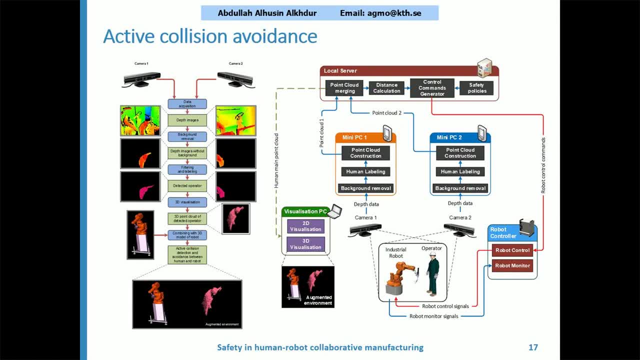 are calculated from the information that are calculated from the information that comes from the robot controller, comes from the robot controller, comes from the robot controller, about the robot, about the robot, about the robot, joint values and basically using that joint values and basically using that joint values and basically using that to, as you can see in the and the figure in 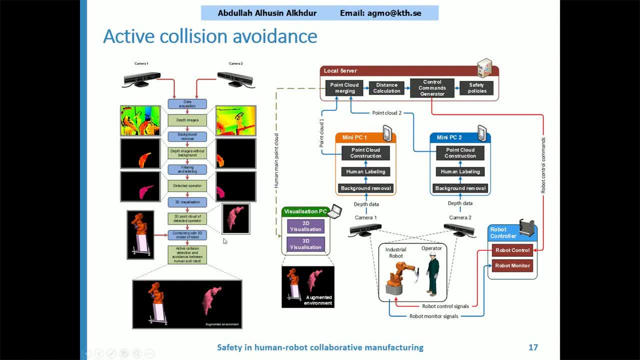 to, as you can see in the and the figure. in to, as you can see in the and the figure in the left side where you, we have these, the left side where you, we have these, the left side where you we have these steps of processing and after that, 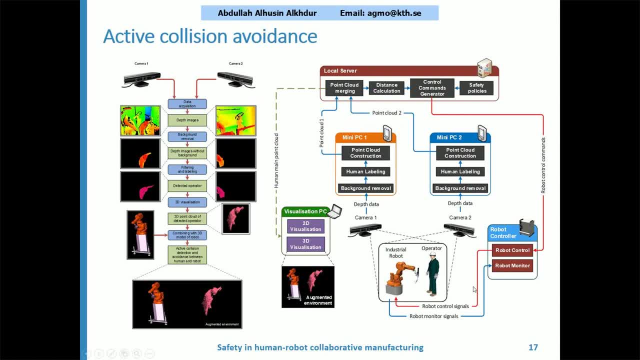 steps of processing and, after that, steps of processing and, after that, controlling the robot, as you can see in controlling the robot, as you can see in controlling the robot, as you can see in the right side, where we have the, the right side where we have the, the right side where we have the signals. 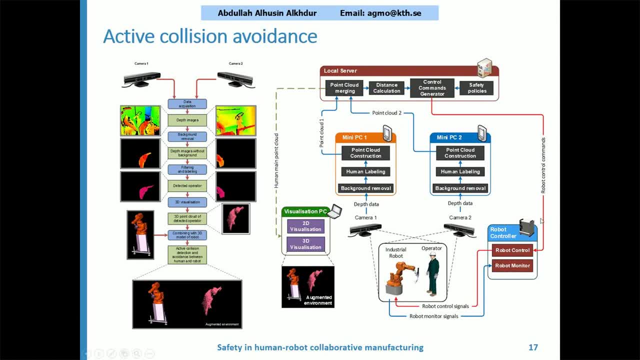 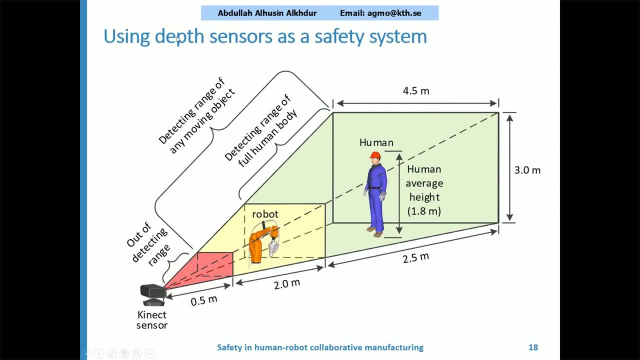 signals. signals as a sensing range for the setup of signals as a sensing range for the setup of signals as a sensing range for the setup of the Kinect. By analyzing this sensing the Kinect, By analyzing this sensing the Kinect, By analyzing this sensing range, we were able to decide where to 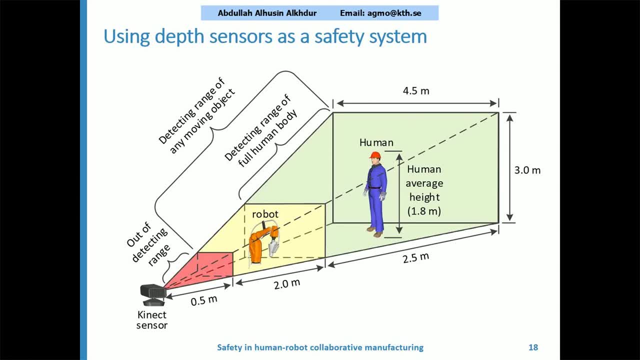 range. we were able to decide where to range. we were able to decide where to put the sensors in the safety system. put the sensors in the safety system, put the sensors in the safety system that we have developed in that case and that we have developed in that case, and 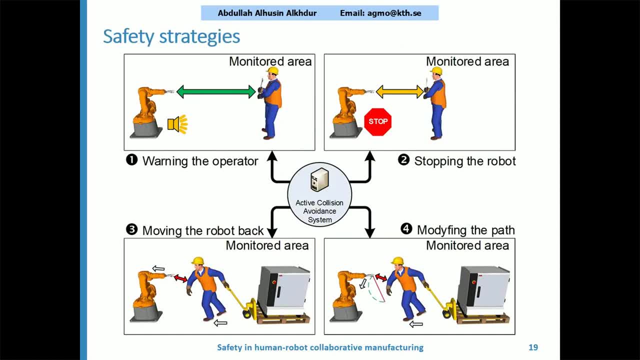 that we have developed in that case and we also be able to define a different. we also be able to define a different. we also be able to define a different safety strategies. the first one is to safety strategies. the first one is to safety strategies. the first one is to warn the operators. so if the operator is 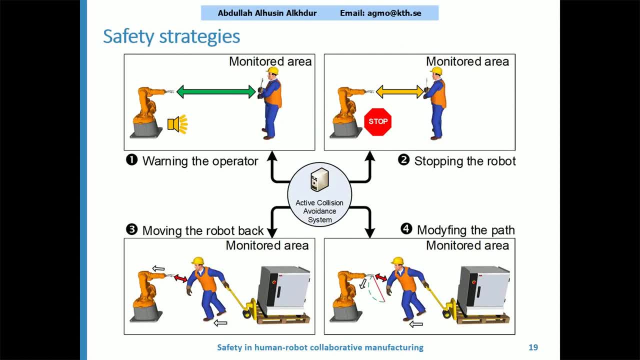 warn the operators. so, if the operator is, warn the operators. so if the operator is within a certain distance, then it will within a certain distance, then it will within a certain distance, then it will trigger an audio alarm. and, in the second, trigger an audio alarm. and in the second, 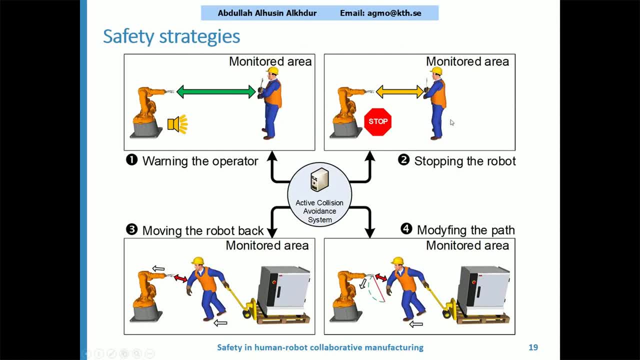 trigger an audio alarm. and in the second, strategy, where to stop the robot, if the strategy where to stop the robot, if the strategy where to stop the robot, if the operator is became very close to the operator, is became very close to the operator, is became very close to the robot. and in the third, 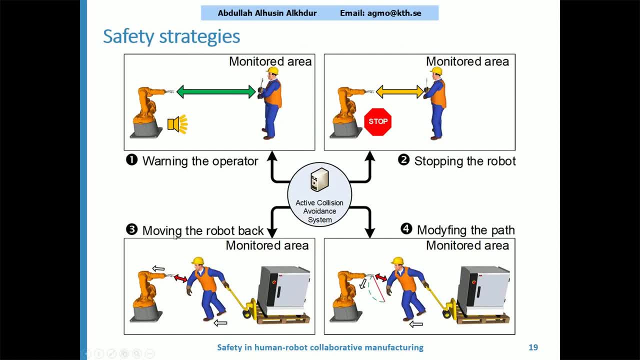 robot and in the third robot and in the third strategy that can be activated, where the strategy that can be activated, where the strategy that can be activated where the robot moves moves away to avoid robot moves moves away, to avoid robot moves moves away, to avoid collision if the operator need to. 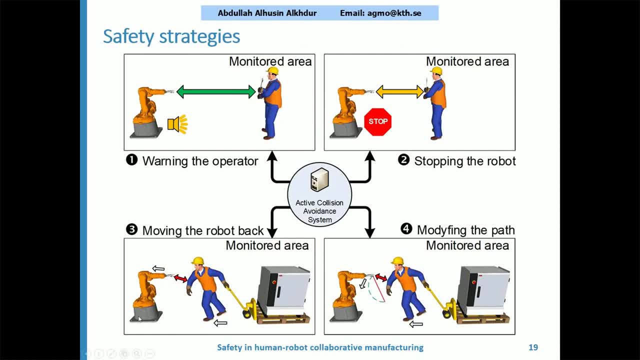 collision, if the operator need to collision, if the operator need to actually go there and be very close to actually go there and be very close to actually go there and be very close to the robot in the fourth strategy, which the robot in the fourth strategy, which the robot in the fourth strategy, which is actually modifying the trajectory of 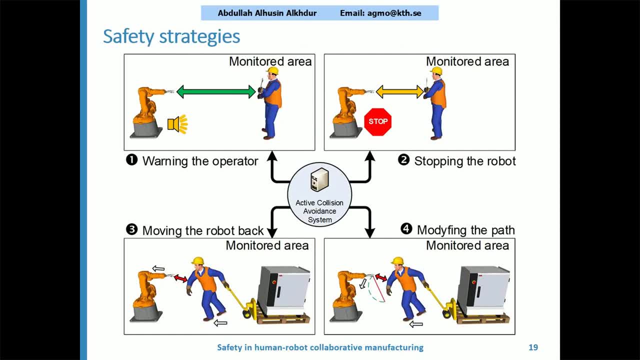 is actually modifying the trajectory of, is actually modifying the trajectory of the robot to avoid collision, the which the robot to avoid collision, the which the robot to avoid collision, the which takes takes takes into consideration performing a certain task that is needed for the into consideration performing a certain task that is needed for the. 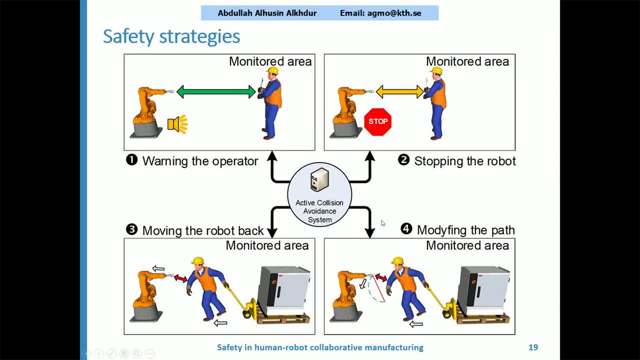 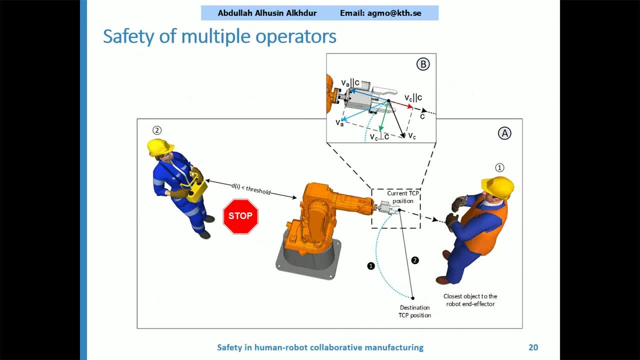 into consideration performing a certain task that is needed for the robot, as well as avoiding the robot, as well as avoiding the robot, as well as avoiding the collision. so, as you can see in the graph here, collision. so, as you can see in the graph here, collision. so, as you can see in the graph here, Victor analysis has been used to. 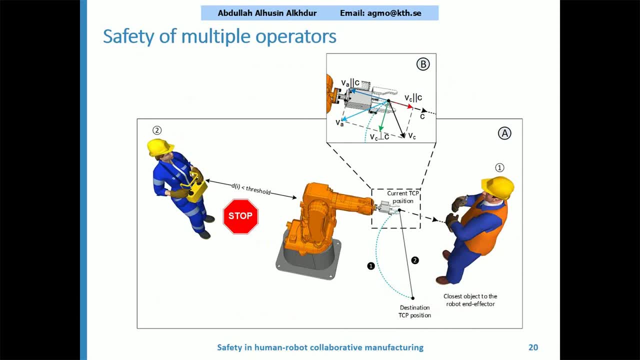 Victor. analysis has been used to Victor. analysis has been used to determine the collision Victor and how determine the collision Victor and how determine the collision Victor and how to avoid it at the same time. fulfill the to avoid it at the same time. fulfill the to avoid it at the same time. fulfill the requirement of the. 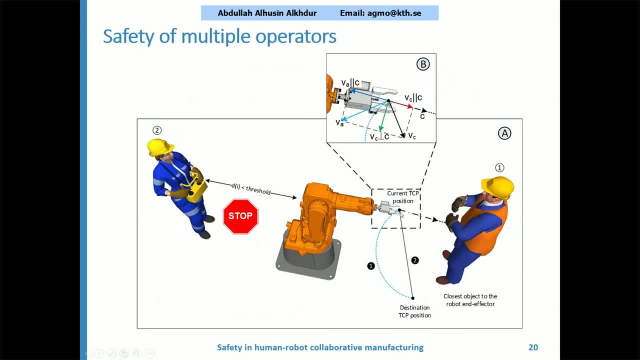 requirement of the requirement of the task. so in the example here, the robot need to task. so in the example here, the robot need to task. so in the example here, the robot need to move in the path which is labeled. move in the path which is labeled. move in the path which is labeled to in the in the lower part of the figure. but 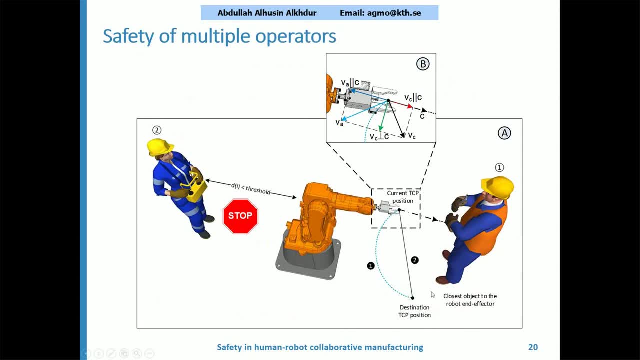 to in the in the lower part of the figure, but to in the in the lower part of the figure, but instead it takes the path number one instead. it takes the path number one instead. it takes the path number one because the operator number one is in, because the operator number one is in. 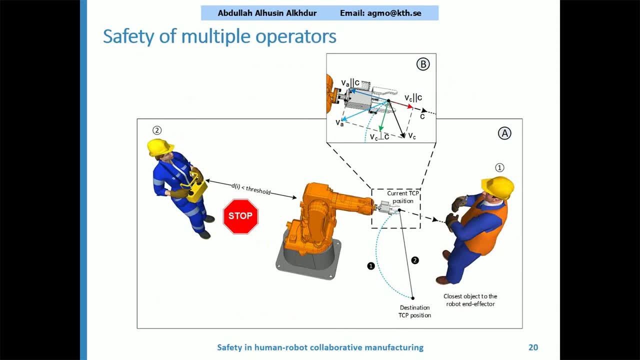 because the operator number one is in the, in the proximity with the, with the, the in the proximity with the, with the, the in the proximity with the, with the, with the robot, and at the same time, we robot and at the same time, we robot and at the same time, we were investigating how to provide the safety.